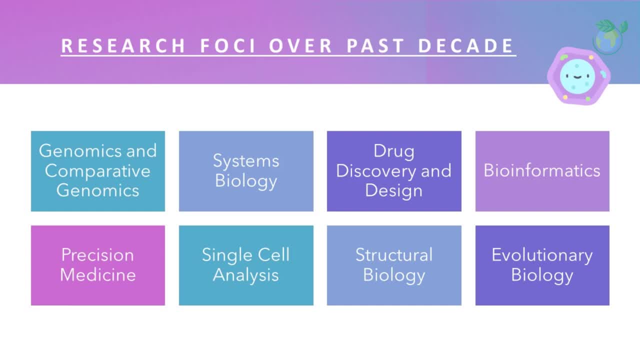 that uses computational methods to analyze and understand biological data. The following are some current research perspectives in this field: Genomics and Comparative Genomics. Studying genomic data of different species to understand the evolution and function of genomes Systems. Biology: Developing mathematical models to understand biological systems and networks and their interactions. 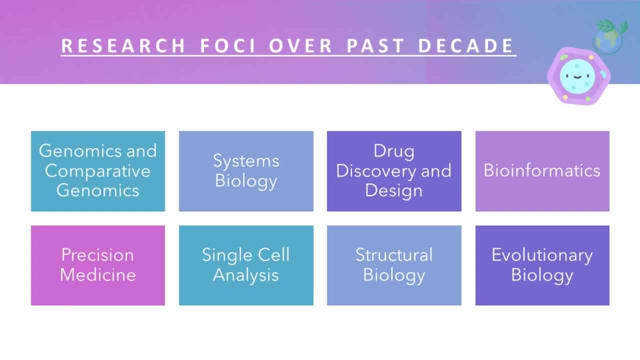 Drug Discovery and Design: Using computational methods to discover and design new drugs to treat various diseases. Bioinformatics: Developing and using computational tools to analyze and interpret biological data. Precision Medicine: Using computational techniques to predict and understand individual patient responses to treatment. enabling personalized medicine. 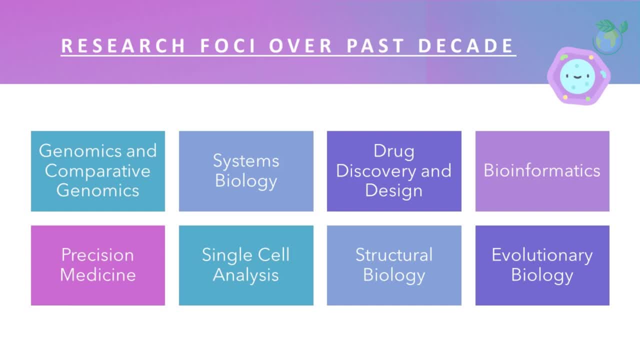 Single Cell Analysis: Analyzing and understanding biological processes at the single cell level, providing insights into cellular diversity and function. Structural Biology: Predictive modeling of protein and nucleic acid structures and interactions to better understand biological systems. Evolutionary Biology: Using computational methods to analyze and understand evolutionary processes and mechanisms. 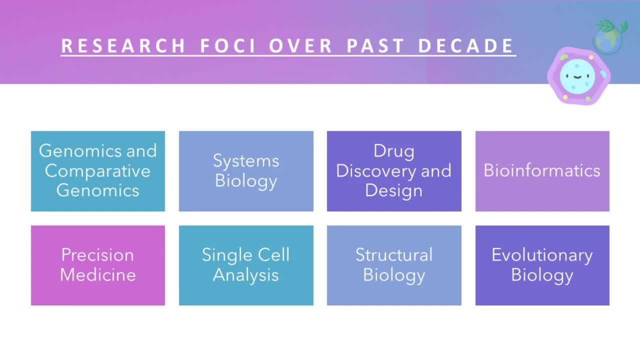 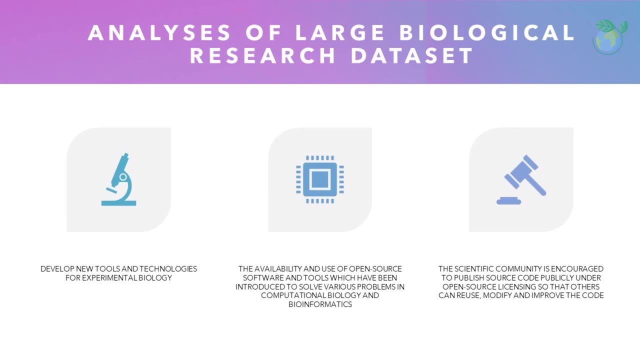 These are just a few of the many research perspectives in computational biology, and the field continues to evolve and expand as new data and technologies become available. Analyses of Large Biological Research Dataset. One of the main areas of research in computational biology is the analysis of large amounts of biological data. 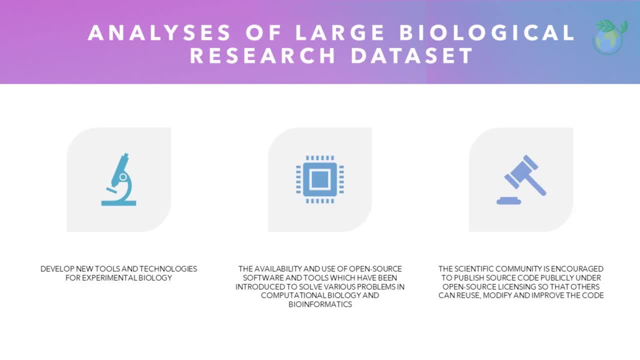 such as data analysis, DNA sequencing data or protein interaction data. This requires the development of sophisticated algorithms and software tools to process and analyze the data. For example, bioinformatics tools are used to analyze DNA sequences, to identify genes, predict protein structures and understand the genetic basis of diseases. 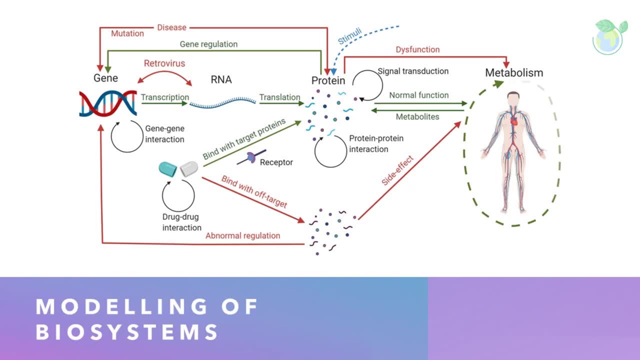 Modeling of Biological Systems. Another important area of research in computational biology is the simulation of biological systems. This involves creating mathematical models of biological systems such as cells or populations, and using computer simulations to study their behavior. For example, computational models can be used to study the spread of diseases, predict the effects of drugs on cells or understand the dynamics of ecosystems. 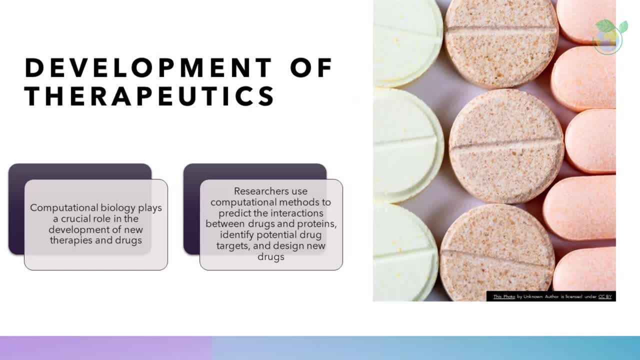 Development of Therapeutics. Computational Biology. Computational biology also plays a crucial role in the development of new therapies and drugs. For example, researchers use computational methods to predict the interactions between drugs and proteins, identify potential drug targets and design new drugs. Tools for Experimental Biology: 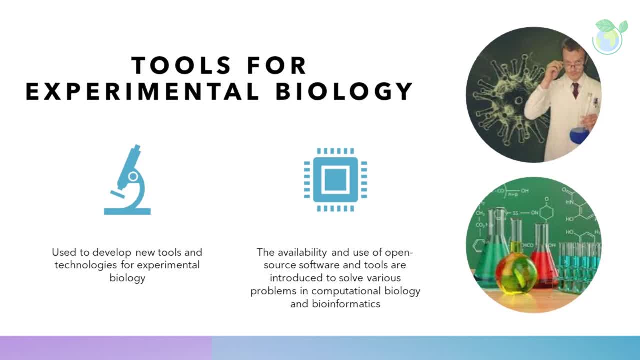 In recent years, computational biology has also been used to develop new tools and technologies for experimental biology. For example, computational methods are used to develop new technologies for experimental biology, And these functional methods are used to design new experiments, analyze experimental data and develop new imaging techniques. 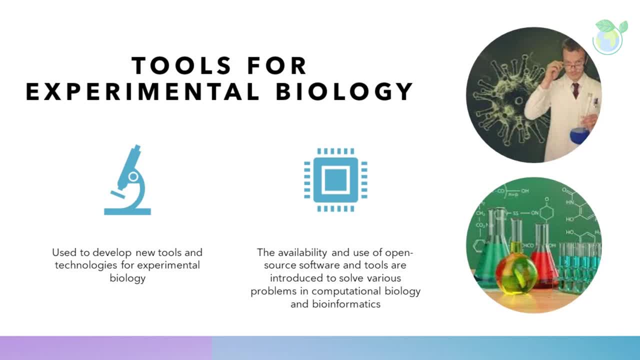 The availability and use of open source software and tools which have been introduced to solve various problems in computational biology and bioinformatics range from simple command-line tools to sophisticated GUI-based applications. The scientific community is encouraged to publish source code publicly under open source licensing so that others can reuse, modify and improve their cryptography problems. 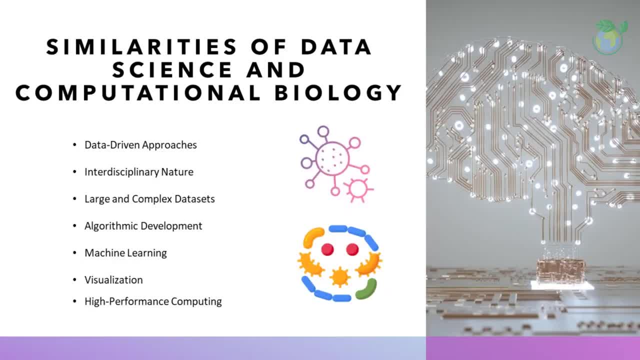 Modification of Biological Systems. modify and improve the code. similarities of data science and computational biology. data science and computational biology share several key similarities, including data driven approaches. both fields rely heavily on data analysis and interpretation to make predictions, draw insights and drive decision making. interdisciplinary nature: both fields bring together expertise from diverse disciplines. 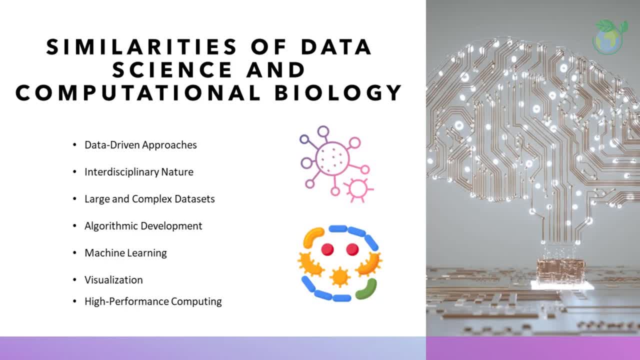 including computer science, mathematics, statistics, biology and others. large and complex datasets: both data science and computational biology require the handling of large and complex data sets, which can range from genomic data to customer purchase history. algorithmic development: both fields provide specific scientific and computational knowledge. require the development of algorithms to extract meaningful information from data, such as: 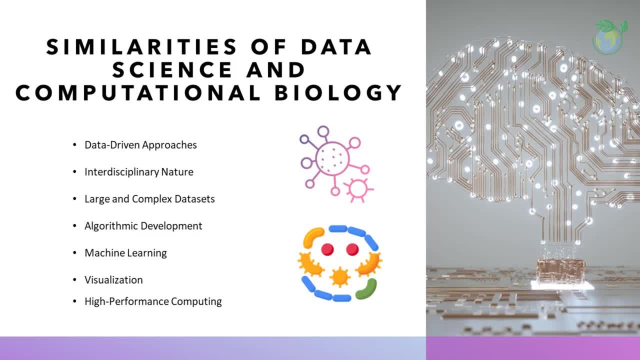 developing models to predict drug efficacy in computational biology or predicting customer behavior in data science. Machine learning – Both fields make extensive use of machine learning techniques to analyze and understand complex data patterns. Visualization – Both data science and computational biology use visualization techniques to present results and insights in an understandable format. 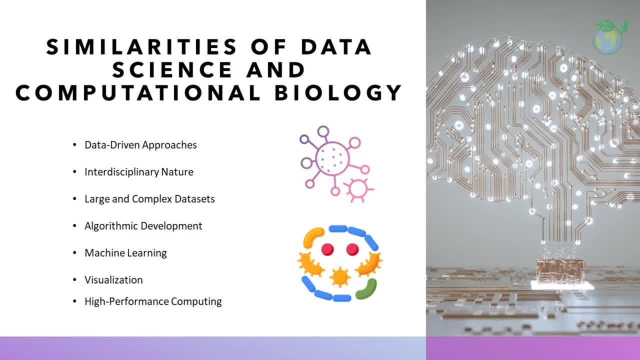 High-performance computing – Both fields often require high-performance computing to process and analyze large datasets in a reasonable amount of time. Overall, the parallels between data science and computational biology are numerous and reflect the growing overlap and integration of computational methods and approaches across many scientific fields. 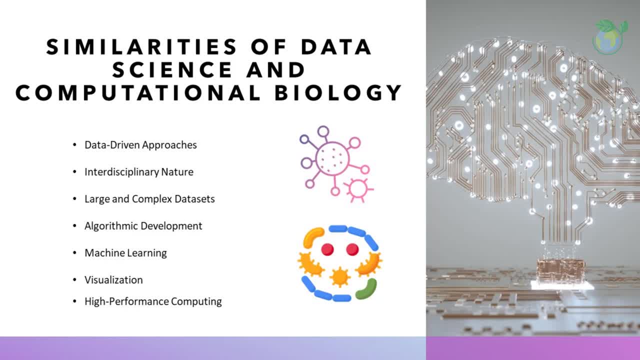 Prospective Outlook – In conclusion, computational biology is a rapidly growing field that is making important contributions to our understanding of biological systems. By combining computational methods with experimental biology, researchers are able to gain new insights into the complex interactions between genes, proteins and cells, which will ultimately 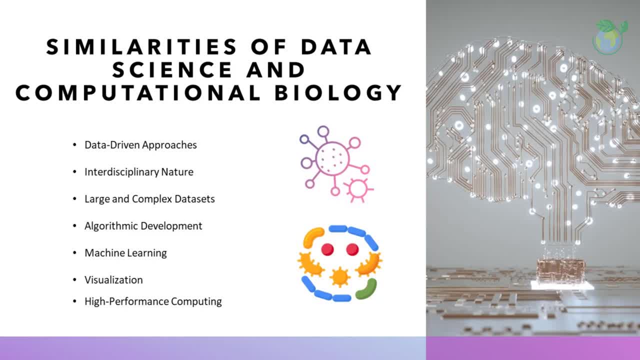 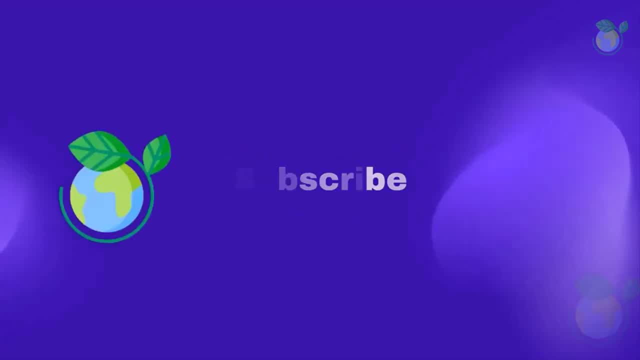 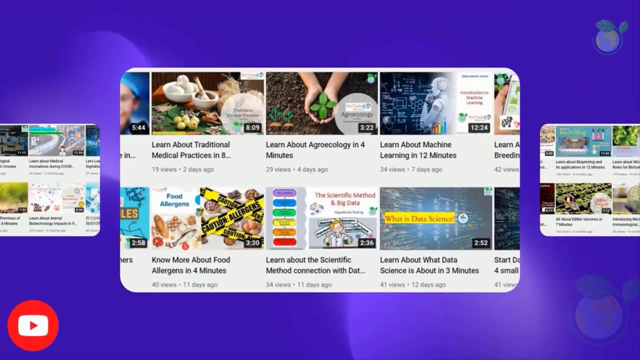 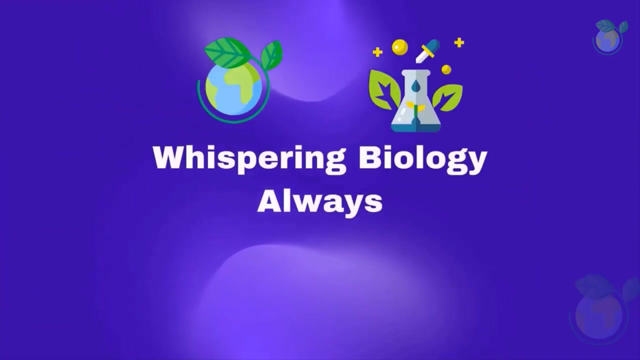 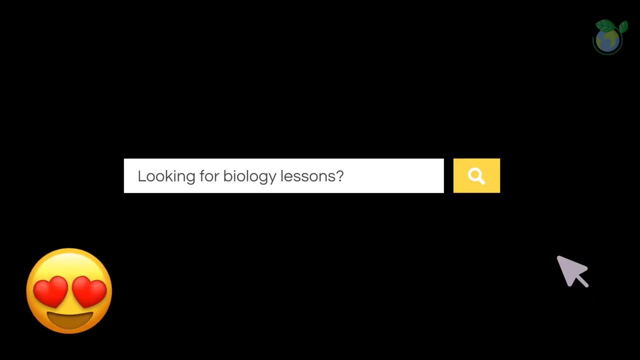 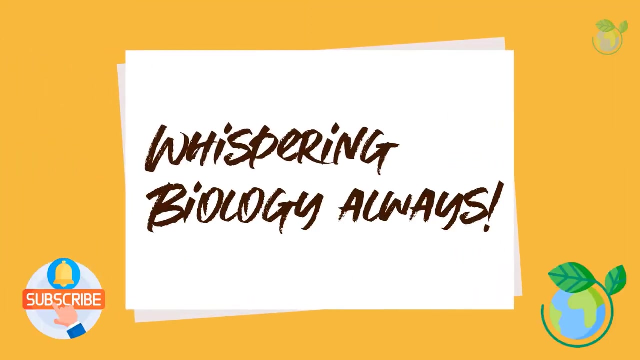 lead to new treatments for diseases and a better understanding of the natural world. To learn more about computational biology, please visit our website at http//wwwhamskeycom. http//wwwhamskeycom.